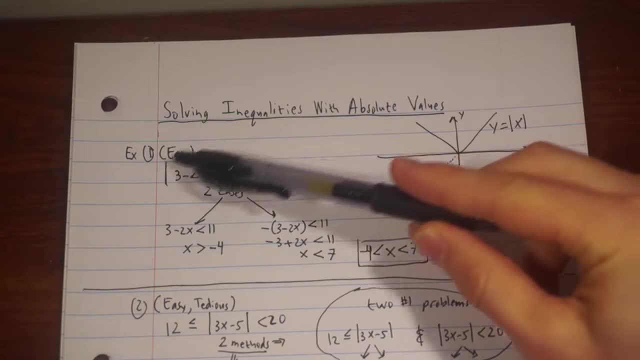 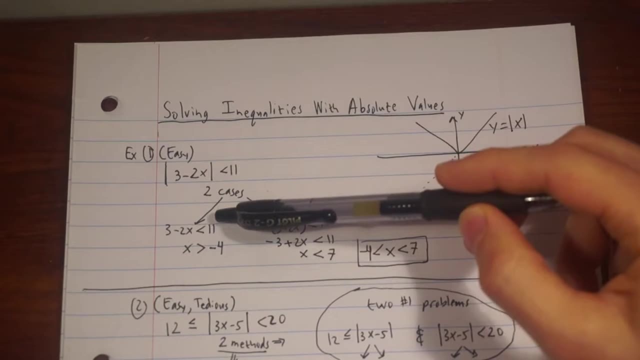 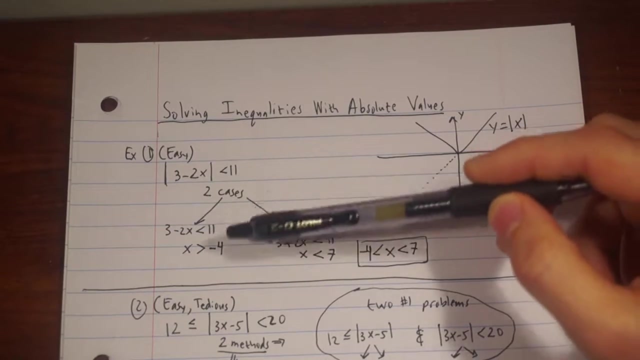 positive or it's zero. So for the first case, we simply drop the absolute value and solve this just like we would in the previous video. And if you move the negative three over, divide by negative two and remember to flip the inequality. x is greater than negative four. that's case one. Now case two means the absolute value is in effect. 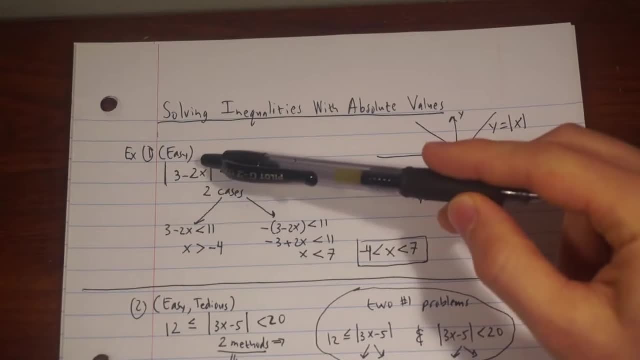 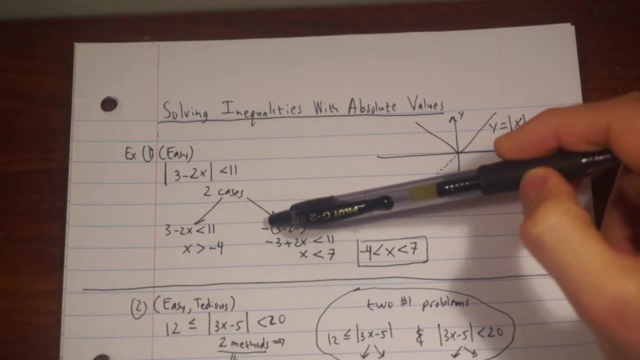 which means this could be negative. So this is negative. then after running it through the absolute value, the absolute value will negate whatever's inside. So that's signified by this minus sign that I've tacked on here. So either you have the original thing or the negative of the original. 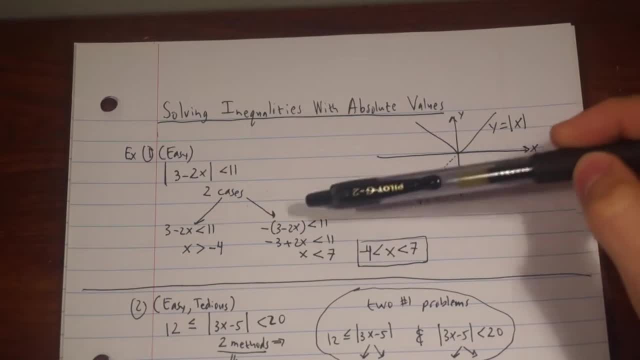 And again, you're going to solve this just like you would normally from what we learned in the previous video. And so, once we solve this, we're going to solve this just like we would normally. So, once we solve this, we'll distribute the minus sign Negative. three plus two x is less than 11.. 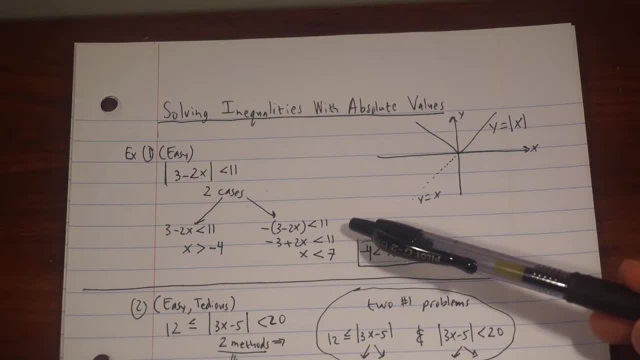 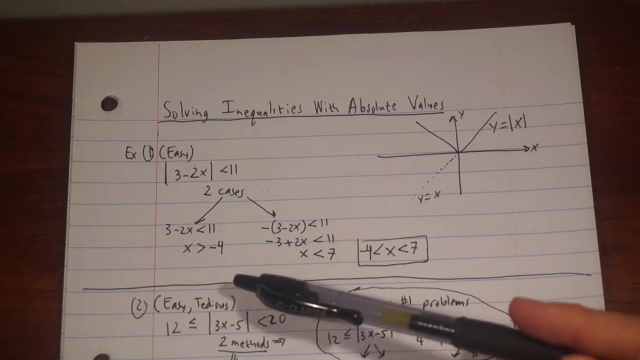 And if you crunch that through, so add the negative three to both sides, divided by two, you should get x is less than seven. So for this one we found that x is between negative four and seven. Now let's go over to a second example. This one's still kind of easy, but tedious. I've only 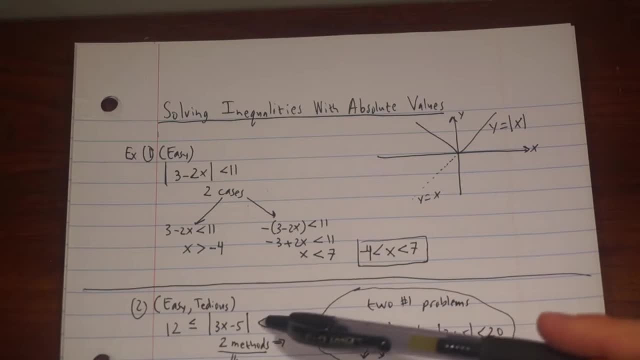 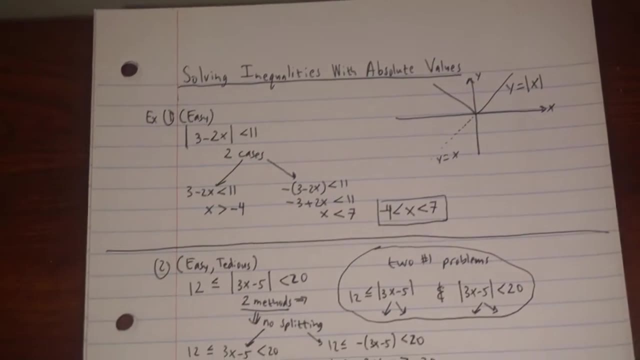 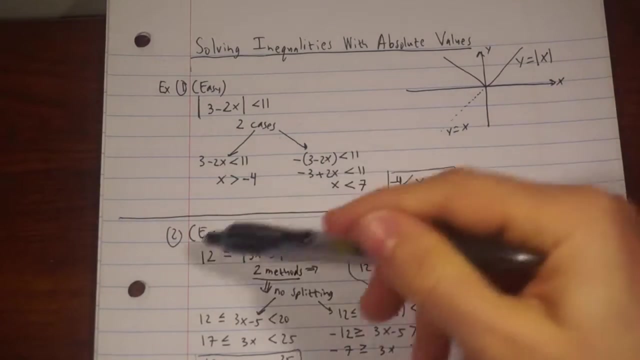 indicated that it's tedious because now we have two inequalities all lumped into one. So there's two ways to do this. The first method is to do this the way we've just done, number one, which is to first ignore this part. So just solve the left half right here and then ignore the 12. 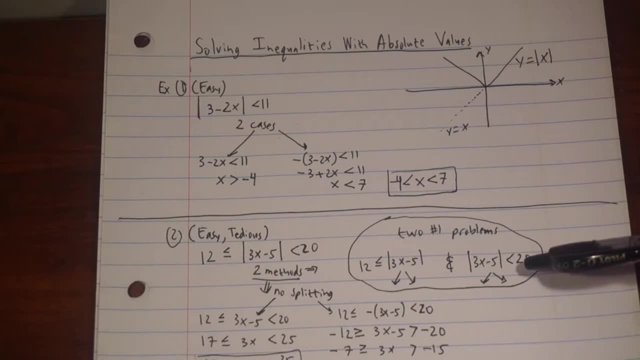 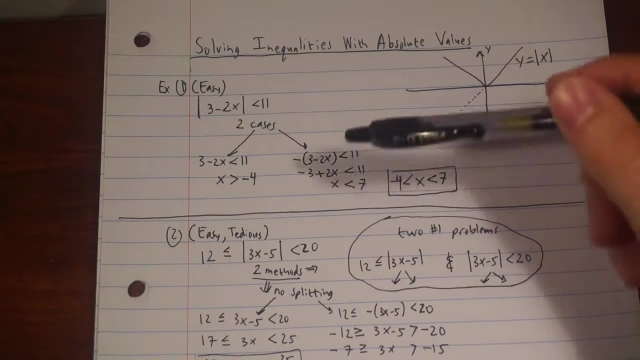 and to solve the right half separately, And then we can combine those answers. I'm not going to do it that way, but you guys can try it. It should be. it should work out very similarly, Just to show you guys kind of a variation on how you can do this all in one shot. So let's go over to the 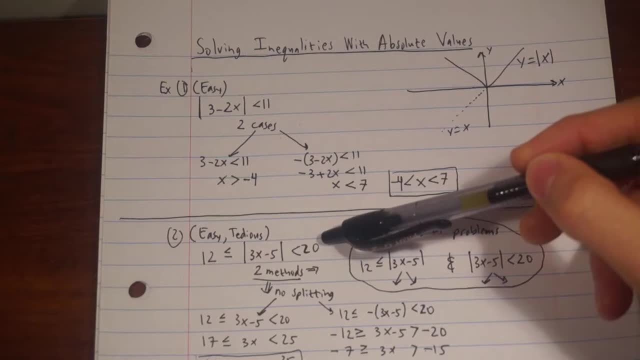 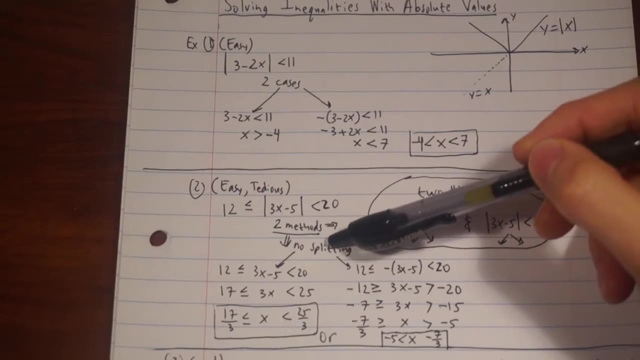 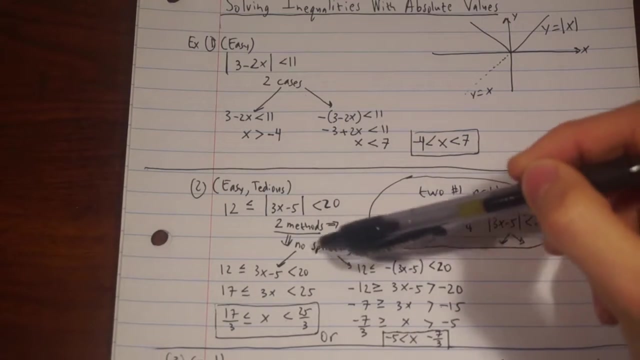 second shot. I'm going to not split this up into two cases, So this is the no splitting version. So there's two cases in the no splitting version, But by no splitting I mean we're going to keep all three parts: the 12, the less than this thing and the 20.. So the two cases are the absolute. 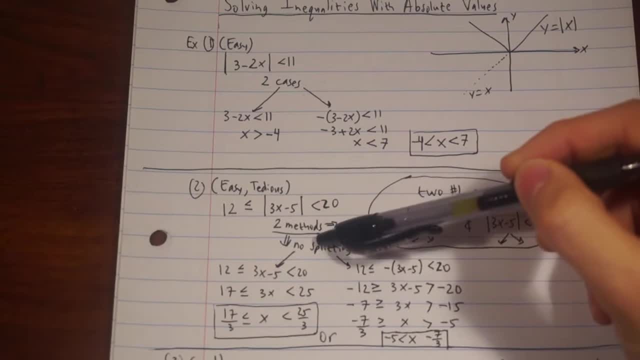 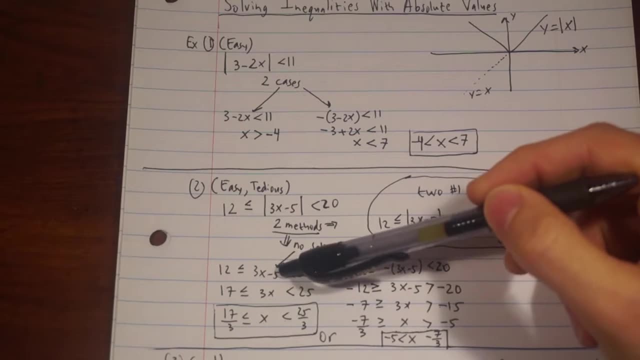 value is an effect or it's not an effect. If it's not an effect, we're simply just going to drop it and solve it without the absolute value. So how are we going to do that? We're going to add this five to one. So we're going to add this five to one. So we're going to add this five to one. 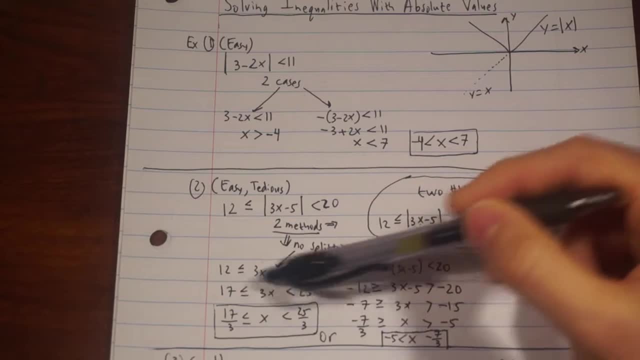 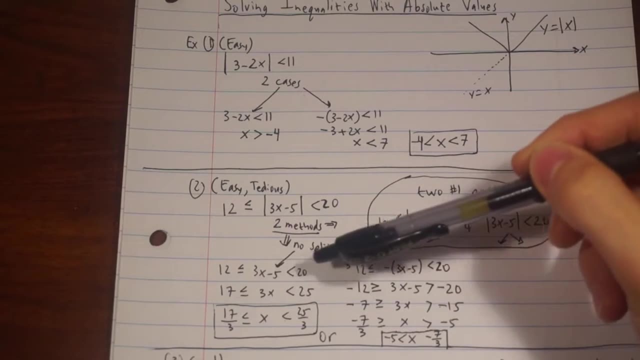 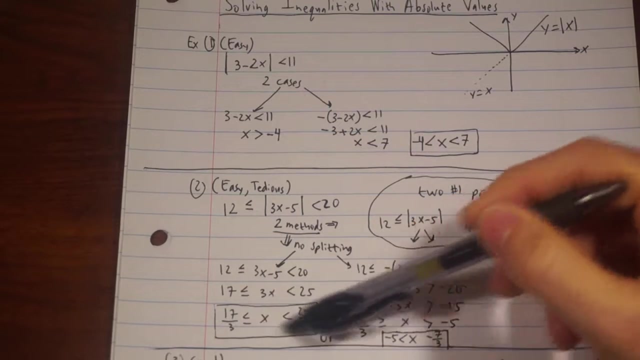 So it's gone from the middle and we've bumped these up by five Now. so we're just almost treating this as like a double equal sign or double inequality, which is what it is. Now we're going to divide everything by three, So that's going to give us 17 thirds and 25 thirds, and 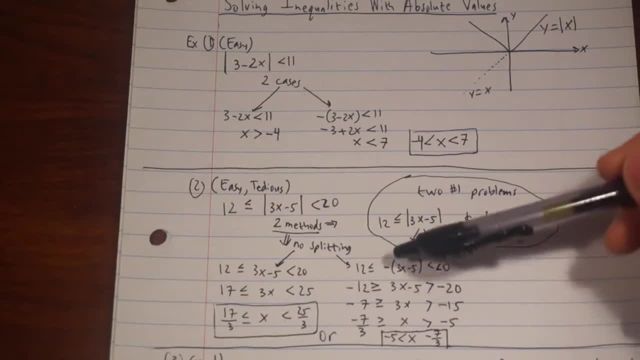 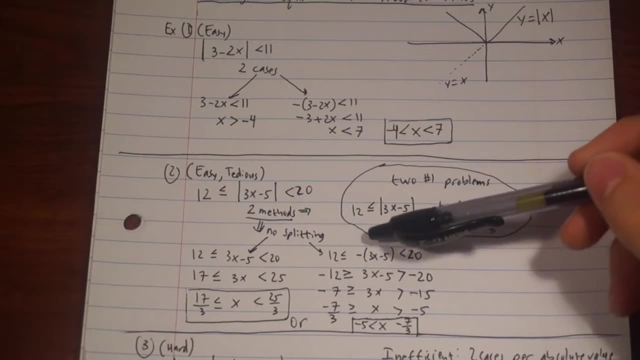 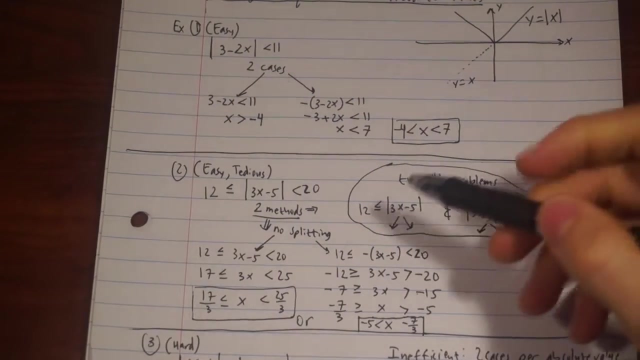 we're done with the first case. Now for the second case. we're going to negate whatever was inside, because now the absolute value is an effect. So now we're going to distribute this minus sign, so that's negative three x. Whoa. Oh no, We're all good. We're all good, Okay. So actually, what I've 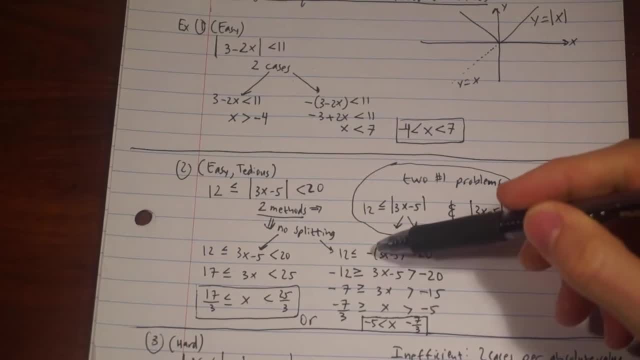 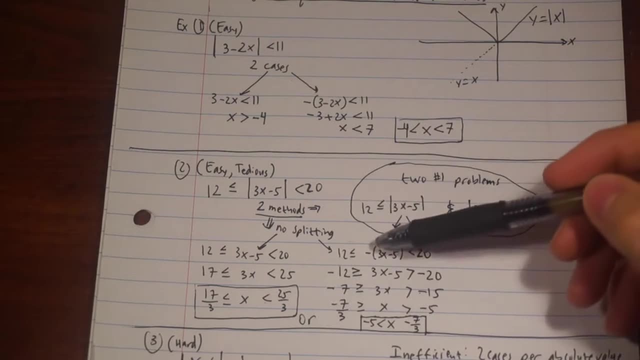 done here is: I'm not distributing the minus sign. I'm annoyed by the minus sign, which is: I first want to divide, or rather multiply, doesn't matter everything by minus one. Now, to do that, I flip the inequality. That's why these signs are flipped over here. So that makes me, that makes there be. 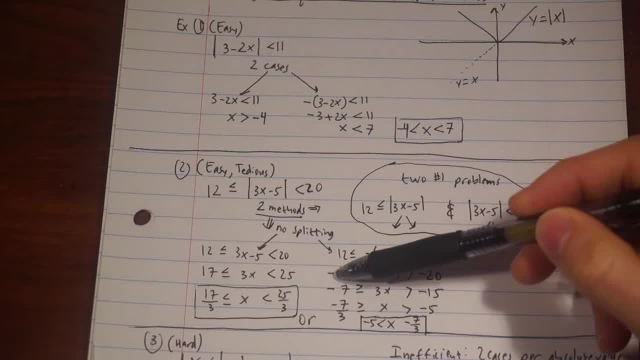 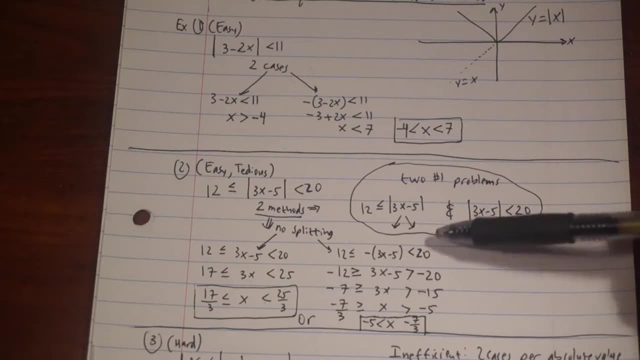 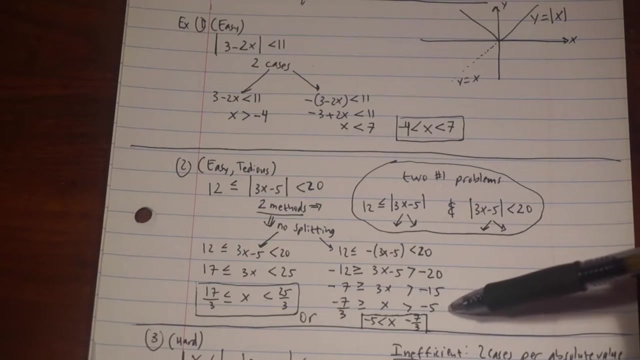 no need to apply this minus to everything. So that's where this negative 12 came from in that negative 20.. These flipped signs. So now we're going to solve this one. We're going to add five to everything, So that's why these are bumped up by five and then divide by three, which is where we get this. 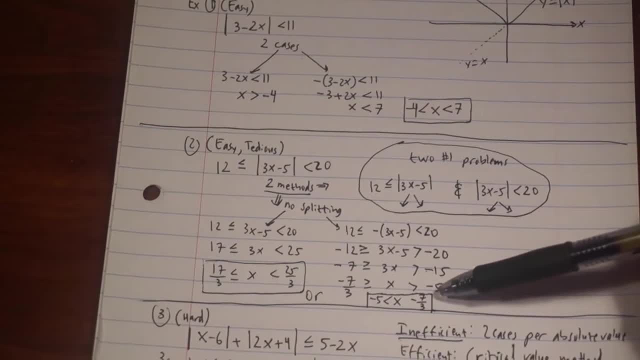 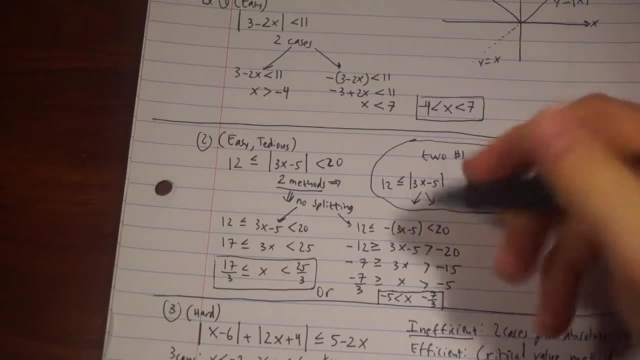 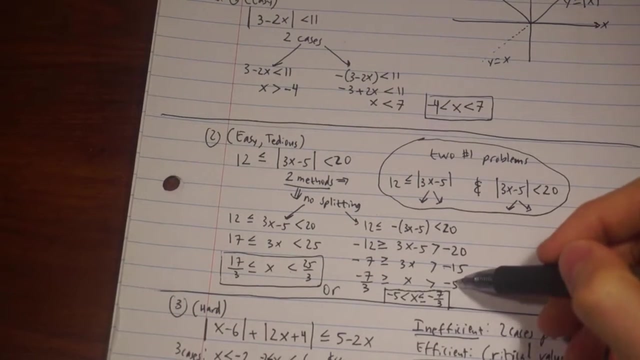 range. So x is between negative five and negative seven thirds. So and he all I've done here is I've simply rewritten it facing the other way. So there's just a missing inequality there, The negative five here on the right, but since it's the lower number, that's why I've reversed the order and put it on. 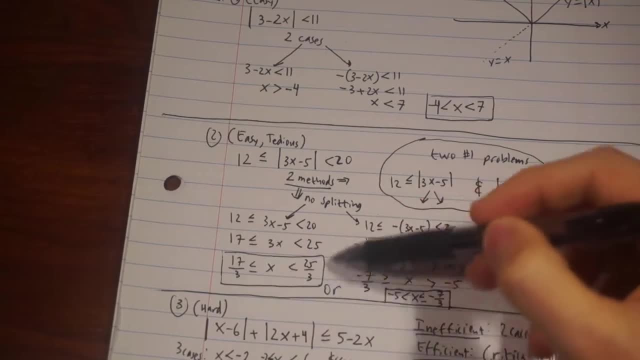 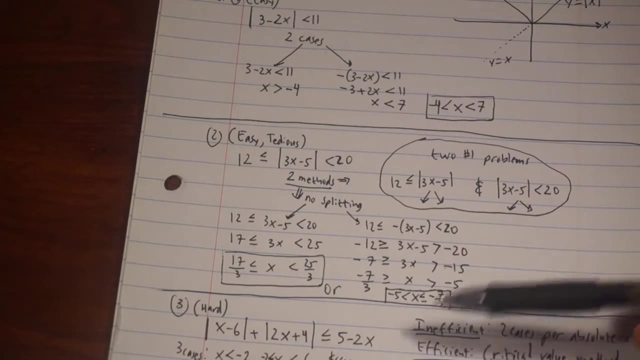 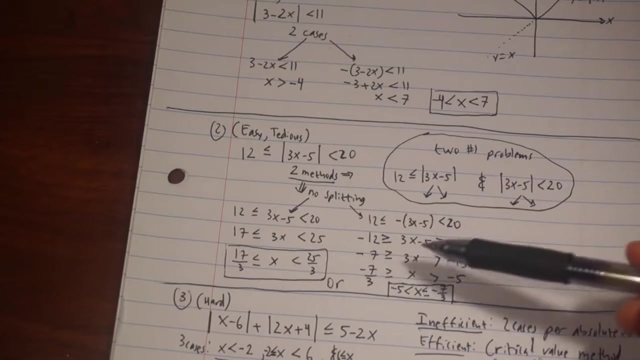 the left here. So we have two solution ranges: either x is between these two numbers or it's between these two numbers. So that's how we can solve this problem all in one shot. Now, had we solved it in two passes, we would have. we should rather get the same solutions. All right, Number. 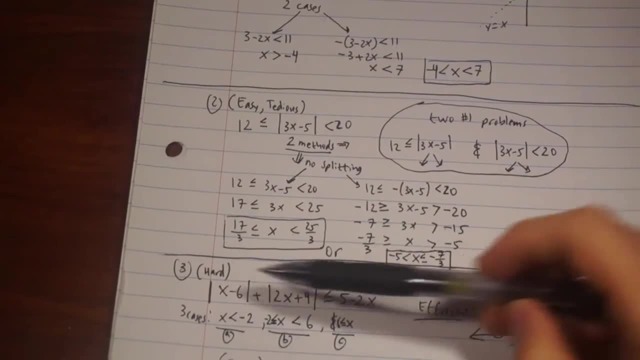 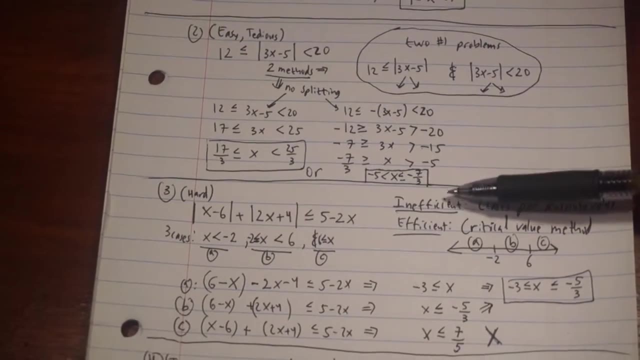 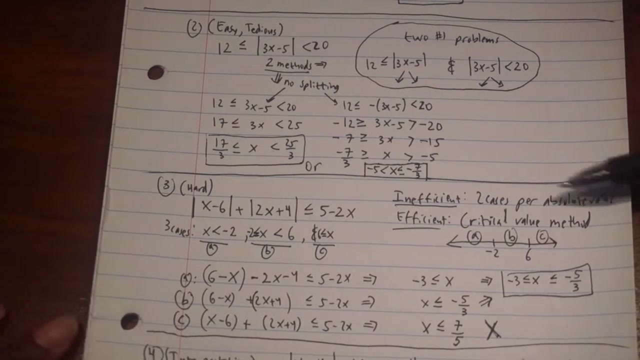 three. So this one's gonna be pretty tricky if you've never seen a double inequality in a problem. So I'm gonna give you guys two ways to do it. The inefficient way, which we won't do, but I'll just suggest it- would be to split this up into two cases per absolute value. In other words, you could treat 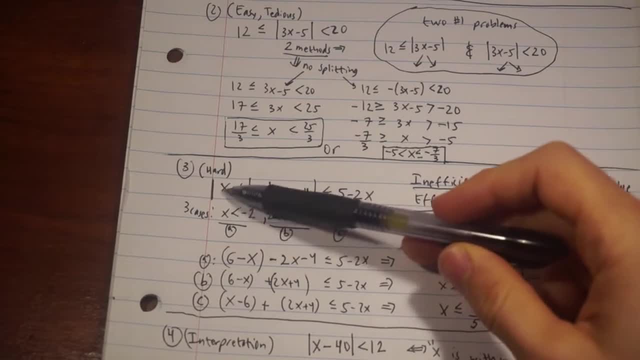 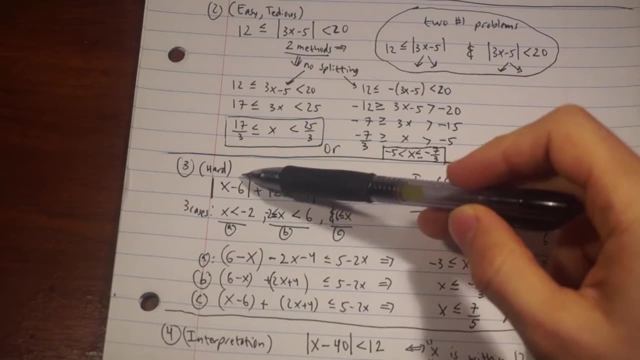 this absolute value separately, And then you'll have two cases: this is an effect, the absolute value is an effect or it's not an effect. In other words, this is either greater than or equal to zero, or it's negative. or this is greater than or equal to zero, negative, And for each of those, 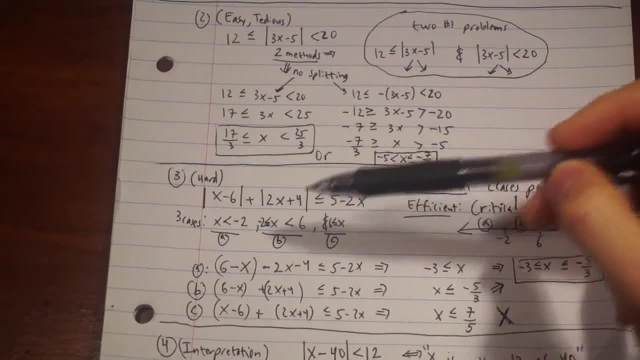 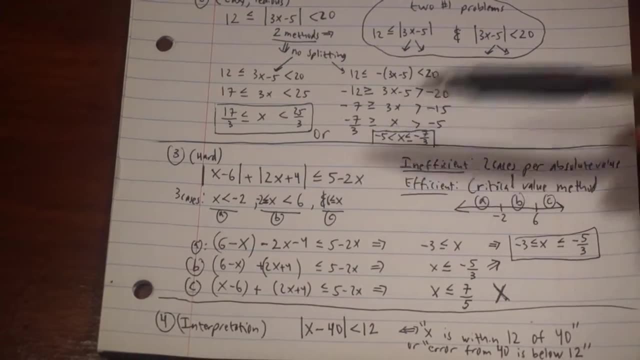 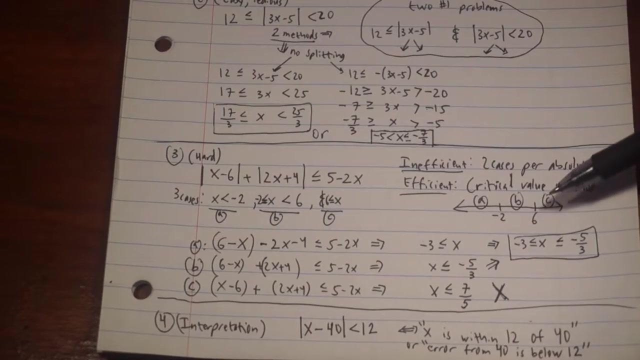 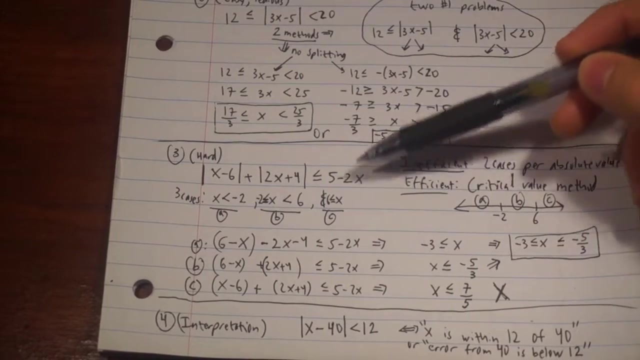 that's two cases per absolute value. Johnny C* quiet, much so. we're going to find a way of doing this using only three cases. How do we do that? This is the efficient method, what I'm calling the critical value method, So we're simply going to look. 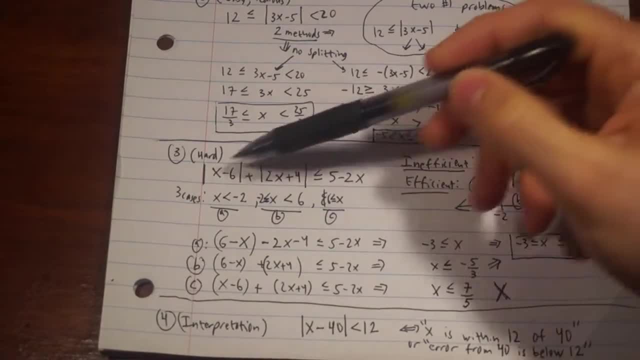 at all the absolute value things. So the x appears here, But there's no absolute value, so we can ignore this part. Number keywordisi value: You think about what value for x makes these parts zero. see that 6 makes it 0.. 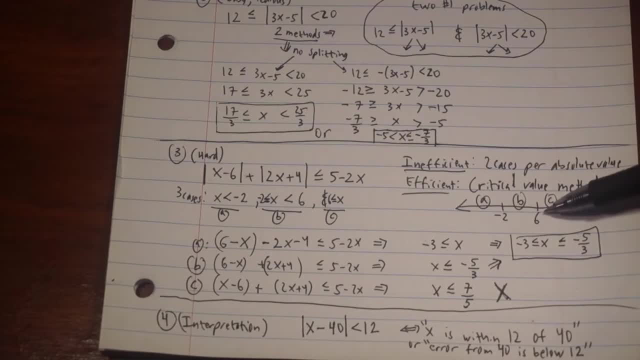 So 6 gets put on one of our critical values And if you try to solve this being 0, you'll find that x equals negative 2 works. So that means rather there being four cases. there's only three cases where x is in this region. 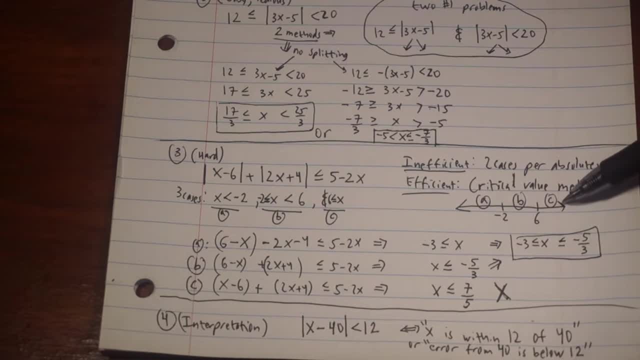 in this region or in that region. Now you just have to be a little careful about whether you're including the negative 2 in this region or that region and the 6 in the b or the c region. So I've defined a, b and c very carefully over here. 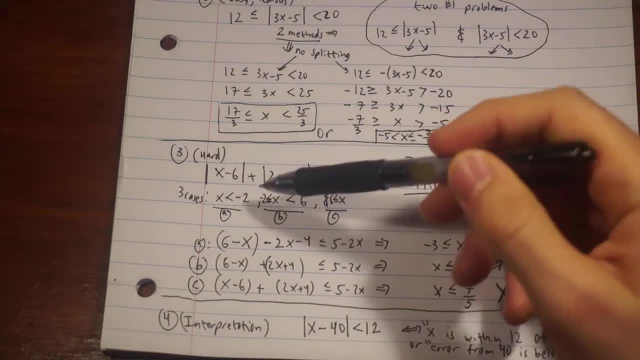 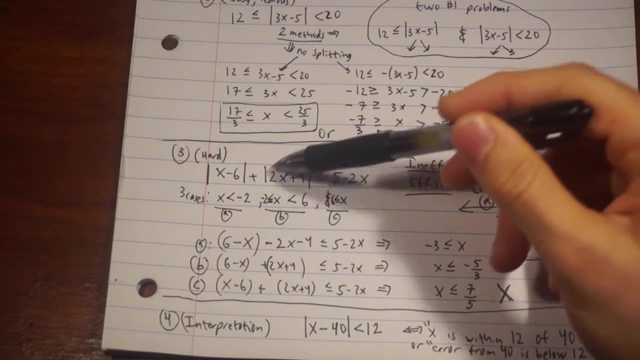 So a is strictly less than negative 2.. Now why did I say strictly? Because if you set x to be less than negative 2, that will cause this to be negative. If x is greater than or equal to negative 2, this is fine. 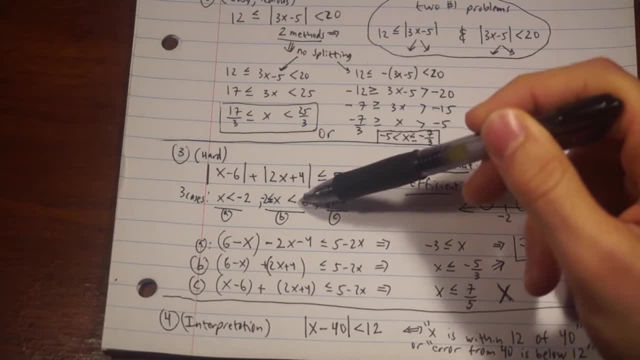 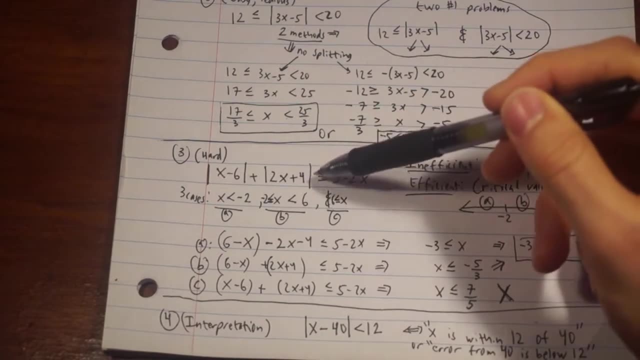 This is going to be 0 or larger, And if it's less than 6, then that one's negative. If x is above 6, then that one's negative. If x is below 6, that means neither of them is negative. 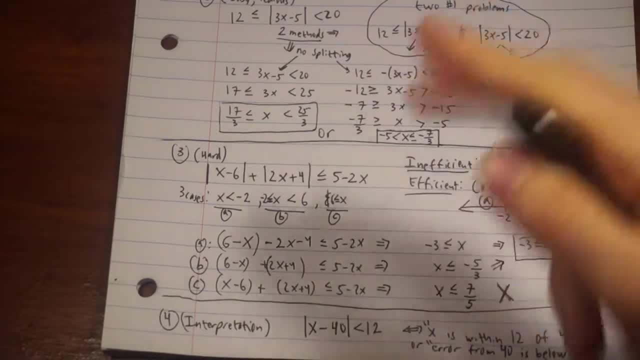 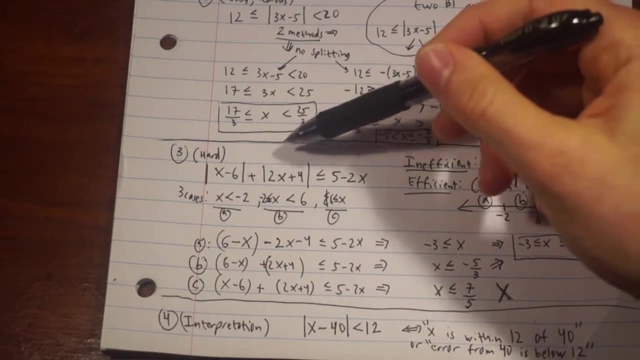 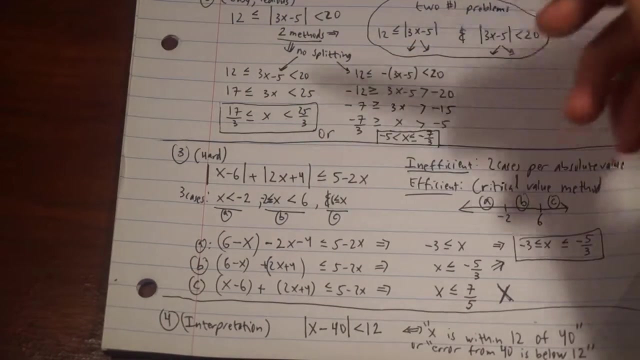 So there's only three cases. You can't have any. which variation? So it's either, to recap, this whole thing is negative, this whole thing is not negative, but this part is negative, or nothing's negative. And if you think about why can't, for example, 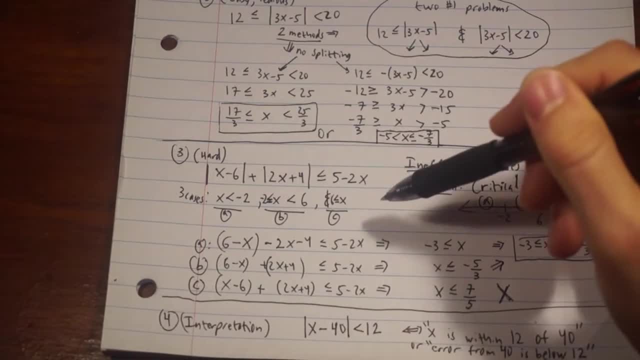 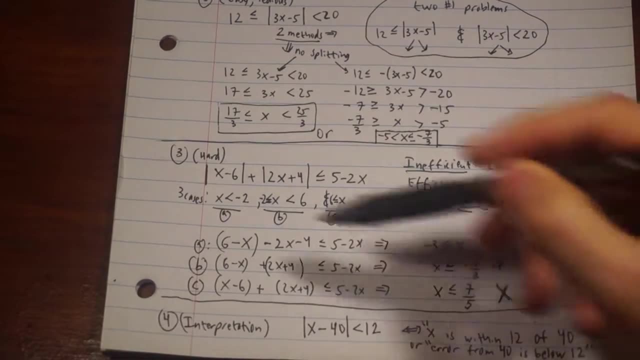 one be negative but not the other. you'll see why there's no fourth case, really OK. So here are three cases, And now I'm evaluating each of the three cases below. So in case A, that means that this part is going to turn out to be negative. 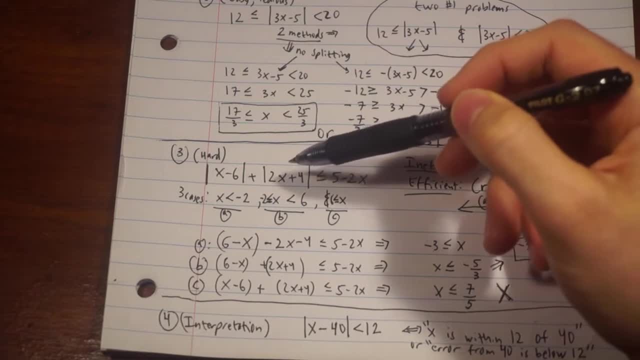 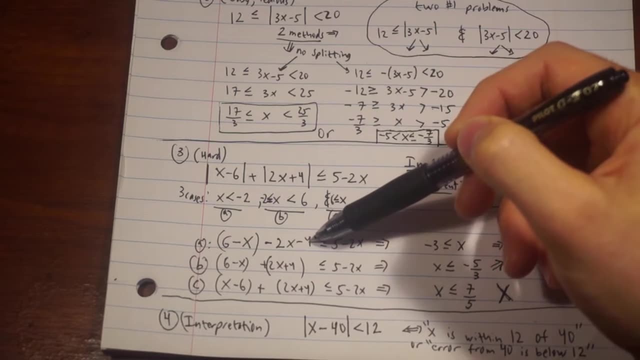 So the absolute value is in effect. So, in case A, what we're going to do is going to have this thing be negated. That's where this negative 2x and the minus 4 came from. Also, if x is below negative 2, this will also. 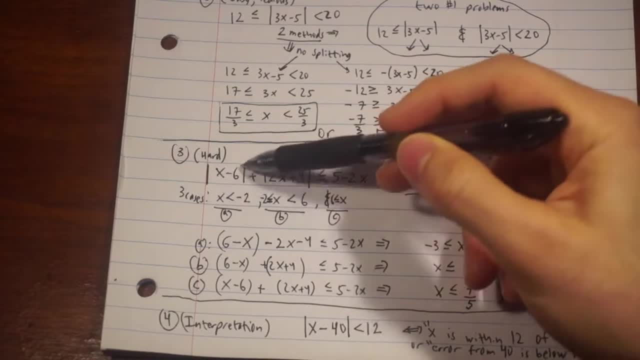 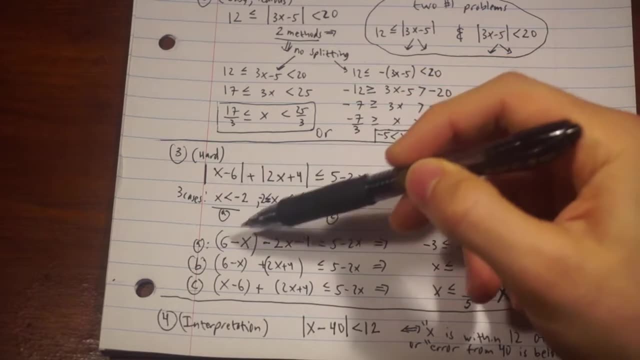 turn out to be negative. So I've negated this whole thing, which is negative of that. But I could also think of it as writing it in the opposite order, which is 6 minus x, If you're having trouble following that. 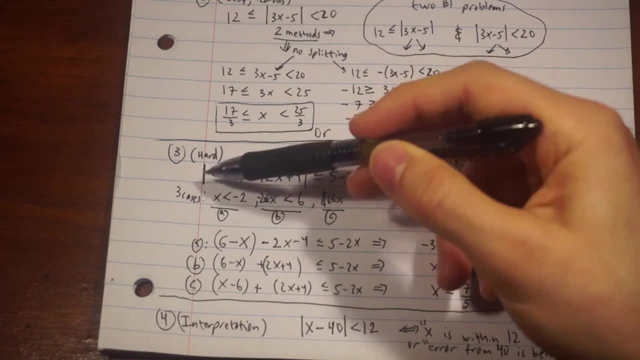 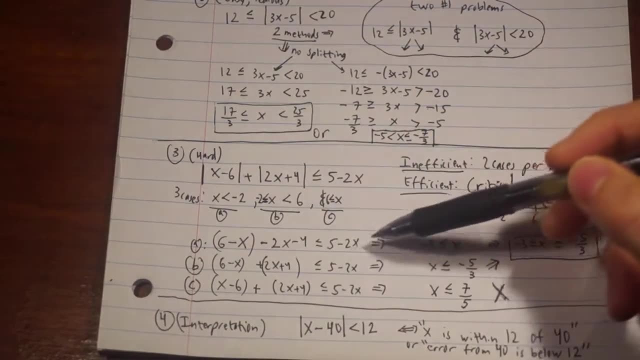 try applying the minus to the whole thing And you'll see that negative x, negative negative 6 is the same thing as that. All right, So that's case A, And now we're going to solve this as we normally would solve an inequality. 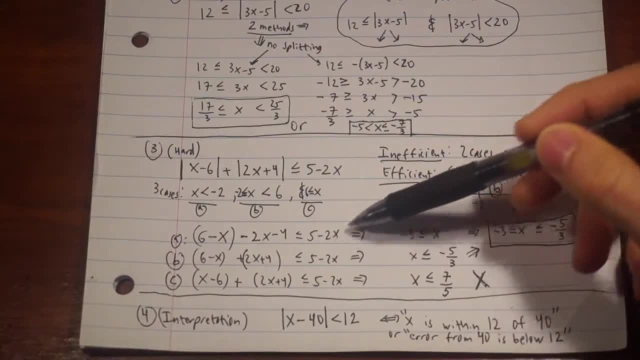 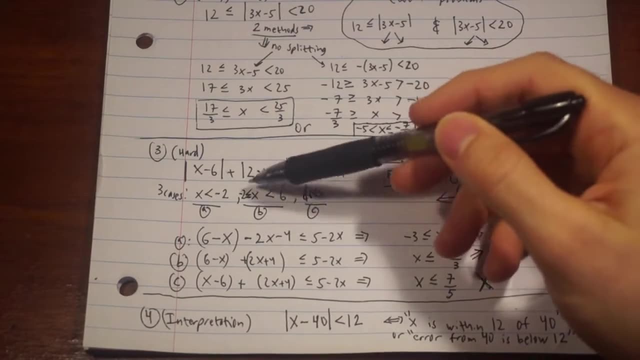 And you'll find that's the solution once you simplify everything over here. Now case B again. we just have to be careful And how to unwrap these inequalities. So in case B, x is between negative 2 and 6,. 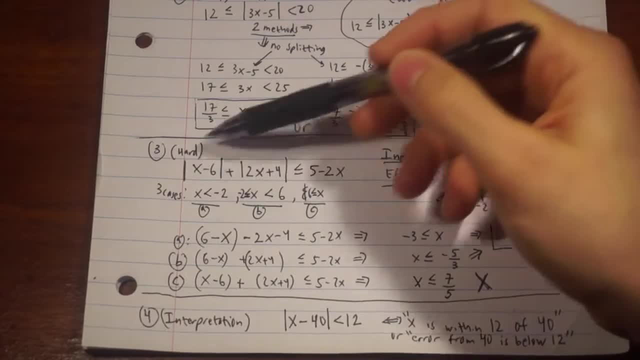 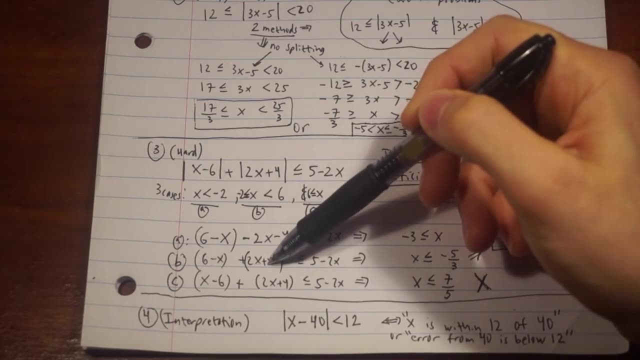 but inclusive of negative 2. So that means that this part will be negative, but this part won't be negative. So that's why this part stays exactly the way it is, But that part is again flipped. And for part C, both of them are unaffected. 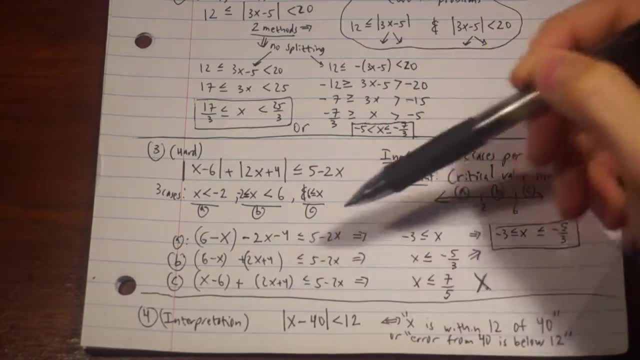 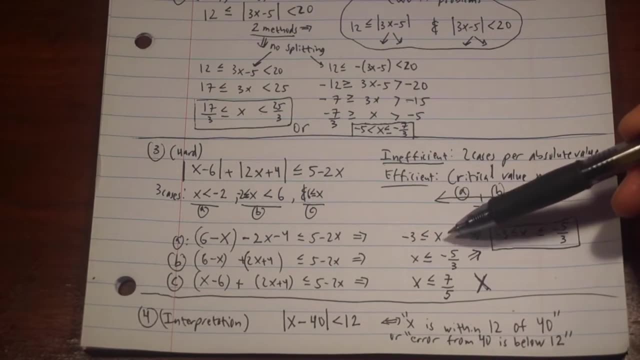 So we literally just drop the absolute value from both of these, And so for all three cases we're going to solve and get these three answers Now. the final step is to remember that, for example, for case C, x is less than or equal to 7 fifths. 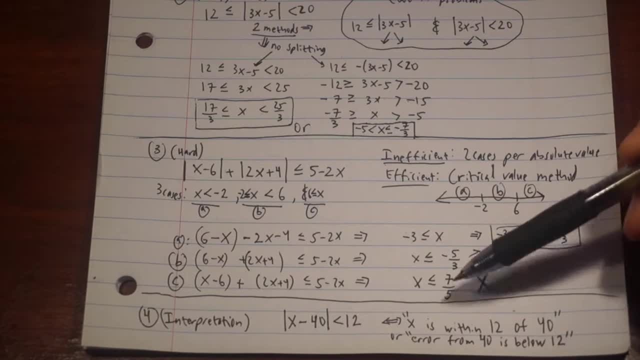 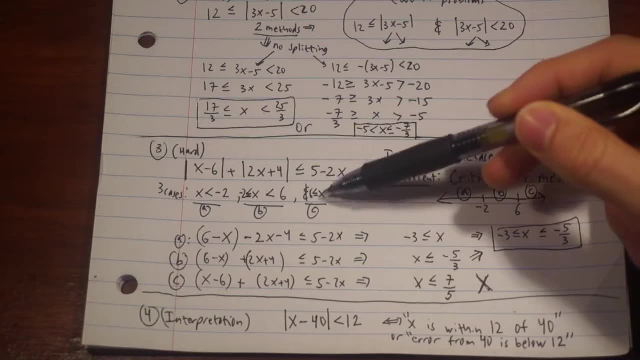 We have to remember that this is not always true. This is only true for case C, which assumes that x is already greater than or equal to 6.. So you can't be greater than or equal to 6 and less than or equal to 7 fifths, which is why we've 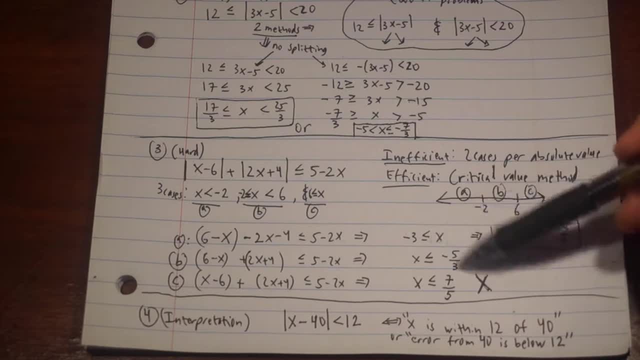 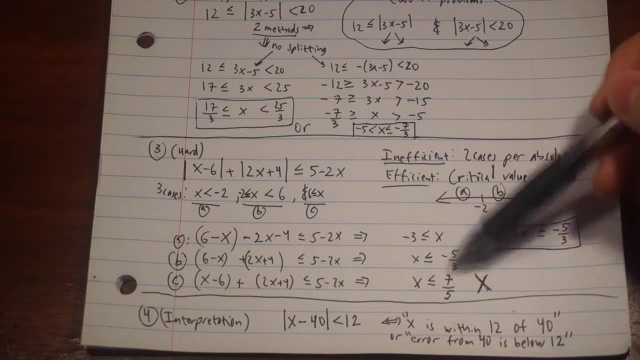 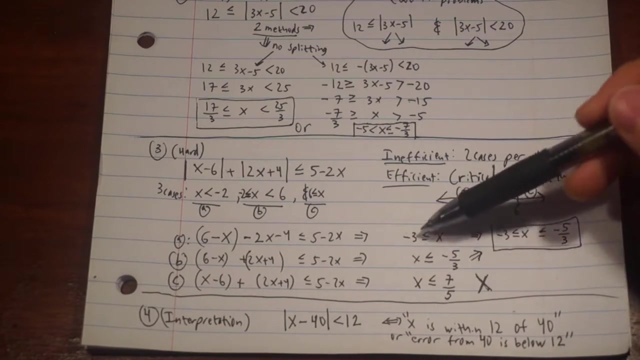 completely rejected this answer. Also, these two answers: they're within the original region, So make sure You further restrict these regions to the original case we're considering. So once you do that, you'll see that there's actually nothing else we have to take into account. 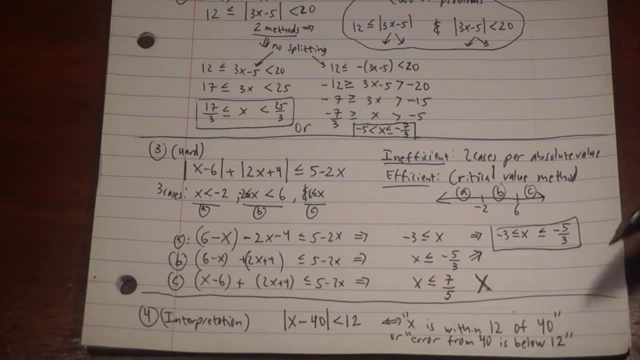 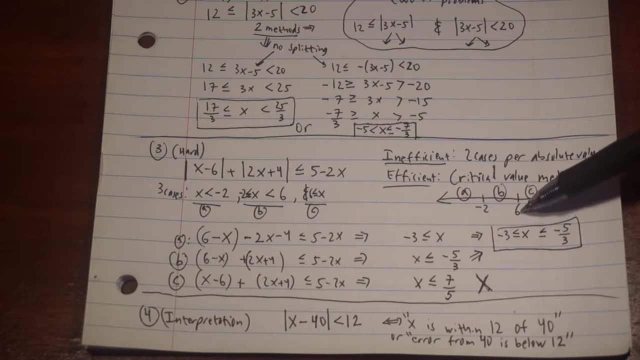 and we can combine these two to get our complete answer. All right. so, to recap, how is this different than the first problem? We found these critical points of negative 2 and 6, and then split the entire problem all in one shot. 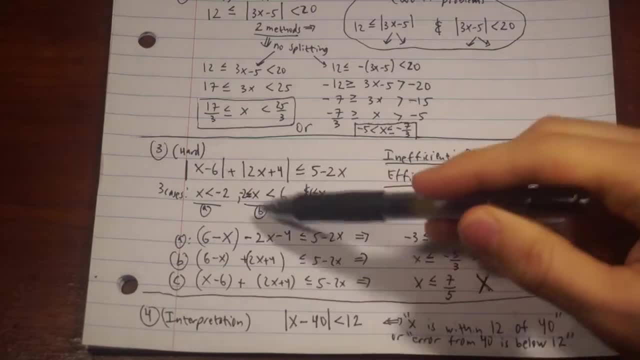 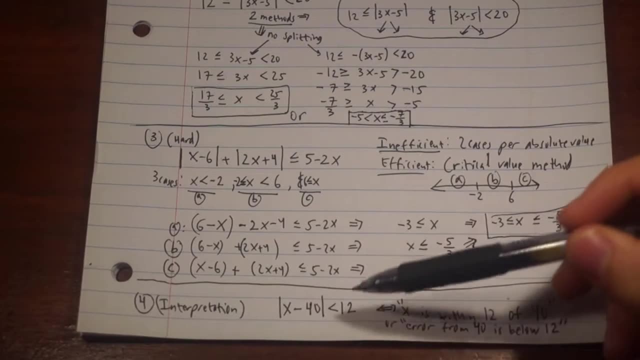 rather than one absolute value at a time, so that we only had to consider three cases, All right. finally, one last point I want to mention to you guys, which is: you might see something like this, And this is just an interpretation question: 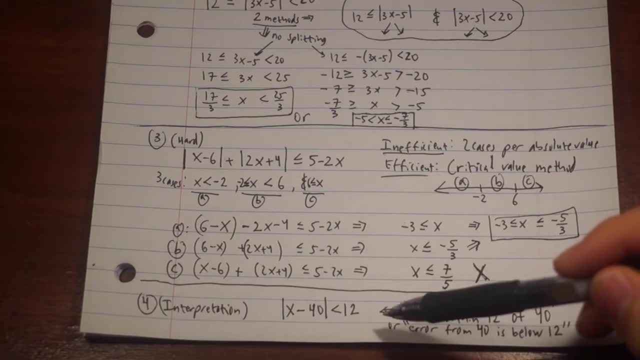 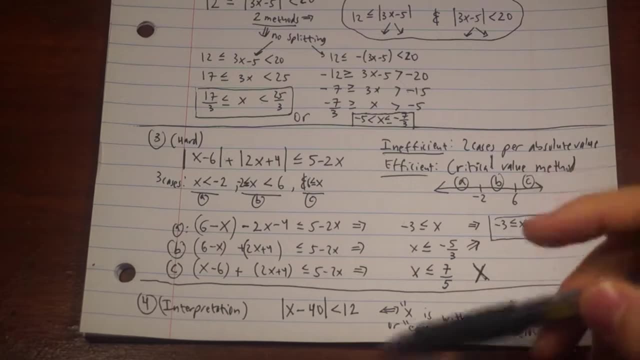 Absolute value of x minus 40,. all of that is less than or equal to 12.. So this is not about how to solve this. If you've followed number one in this video, you should be able to solve this. This is about how do you interpret this. 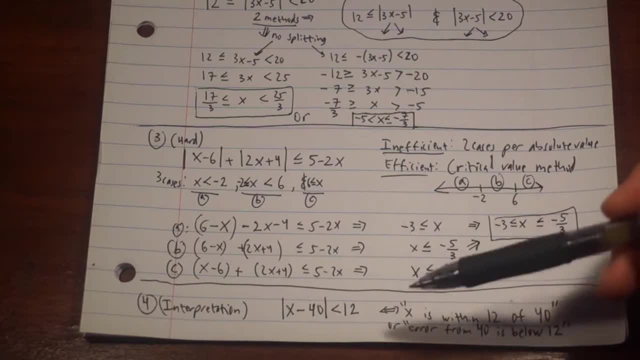 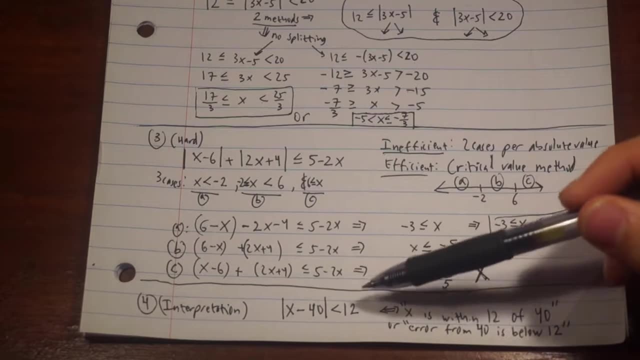 So if you've ever been in a physics lab or a chemistry lab, or it doesn't matter really anything- there's just an intuitive way to understand this, rather than just through algebra. You could think of this as saying x is within 12 units of 40,. 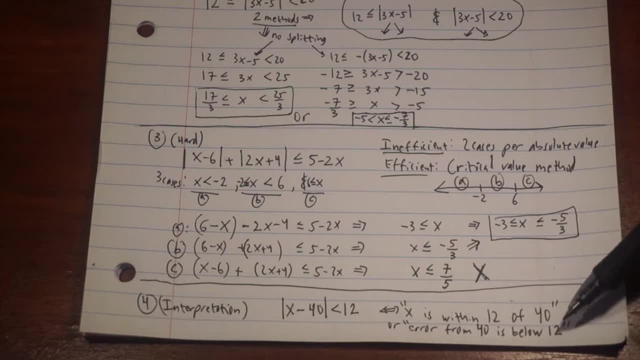 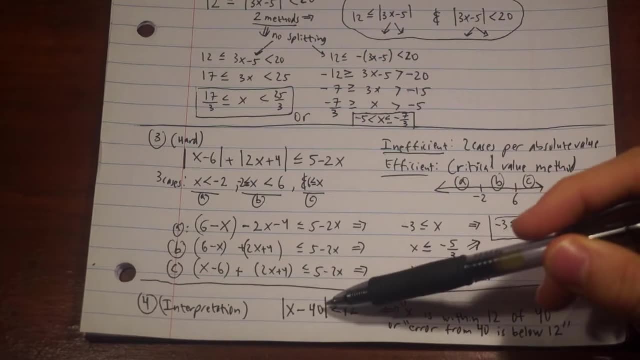 or the error from 40 is below 12.. So, for example, let's say you want to create a desk and the perfect size desk is 40 inches wide. However, your person, the guy that's making the desks, is a little sloppy. 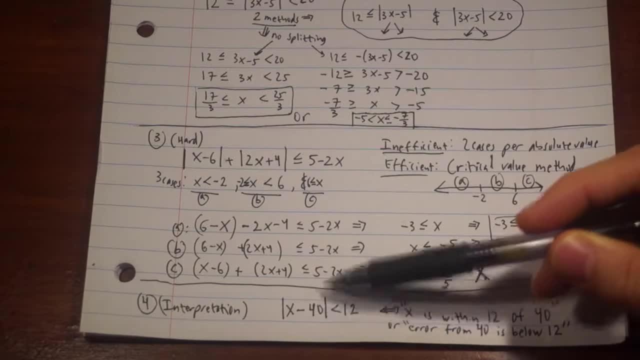 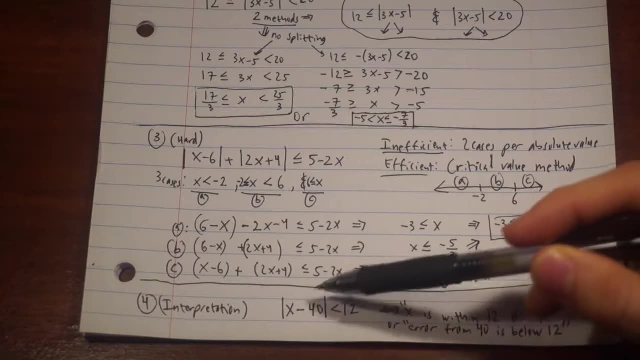 So sometimes they're 47,, sometimes they're 38. They're always around 40, but they're rarely perfectly 40. So this is another way of saying that as long as this error is below 12, you're fine. So the absolute value can be thought of as saying the error. 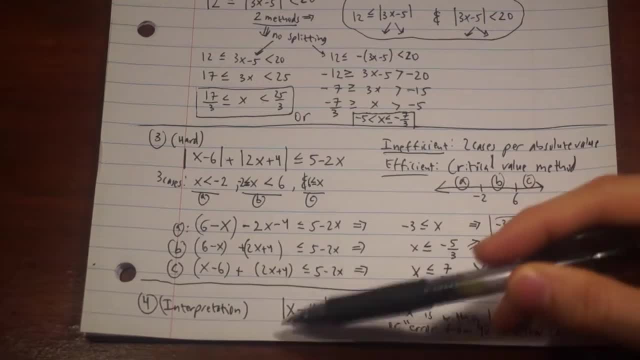 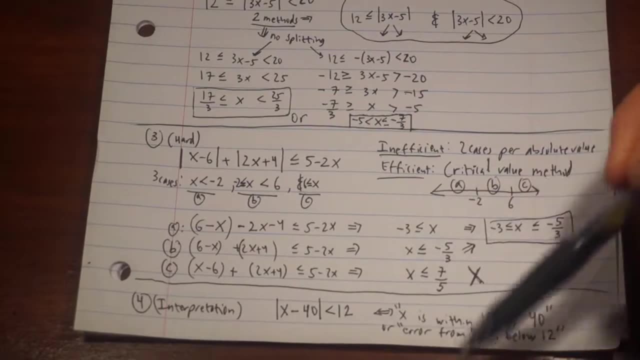 Because if it's above or below it, you don't care, It's just going to take the positive value. And so when you see things like this, a lot of people know how to solve them, but they have no intuition behind what this means.